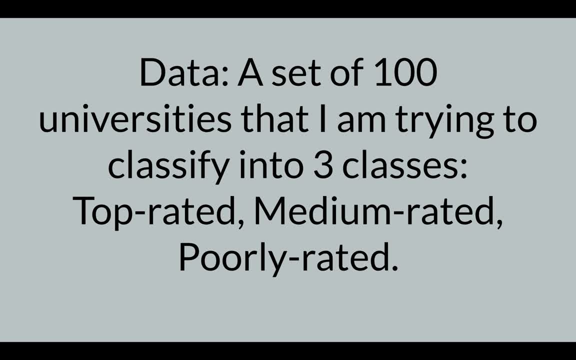 and poorly rated university, and my data contains a number of different features or characteristics about these universities. for example, what is the tuition fee of each each University? where is it located? what is the placement percentage? what percentage of people are graduating every year? what kind of research is happening? what kind of professors are the professors are? 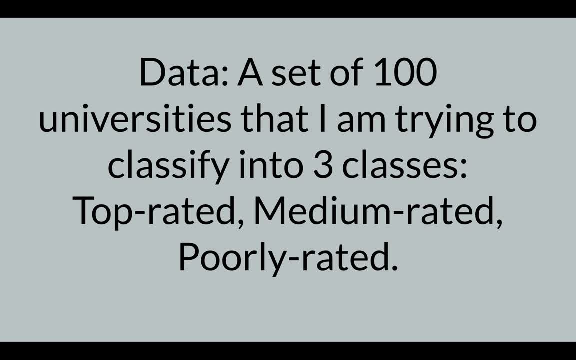 there. you know so a lot of data like that scholarship, and then I feed this data into my decision tree algorithm, and what my decision tree algorithm will try to do at that point is to find which features out of all of these features, or which characteristics out of all of these characteristics that are present. 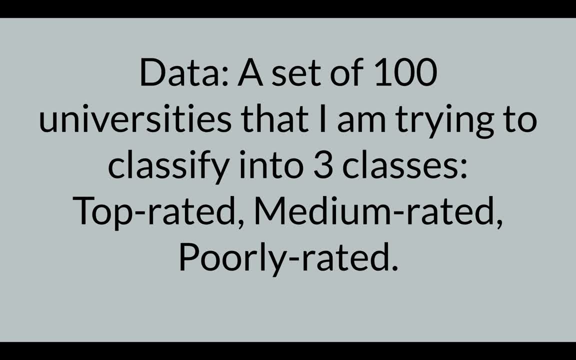 in my data, set against each university, is really helping to classify my data as cleanly as possible into the three different classes. so it will search for the best features which will enable the algorithm to do this task of classification right. so the features that the decision tree will 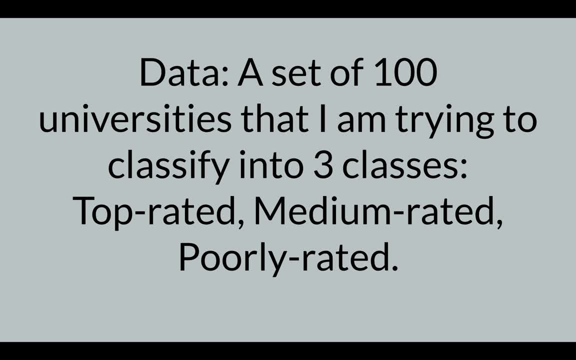 choose will be used in the splitting criteria. so, if you remember the decision tree, how decision tree looks like, it's kind of a flowchart and at every node it splits into two or more nodes. so that splitting criteria, the criteria using which the you know, the higher level depths of the decision tree, will be. 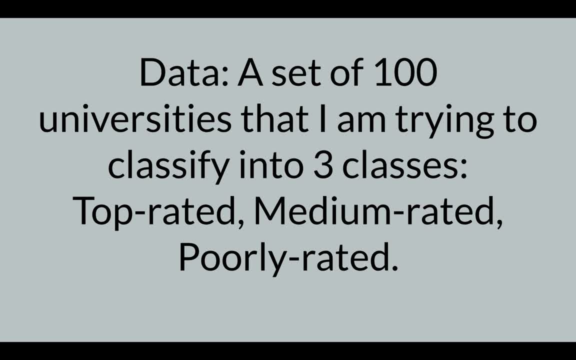 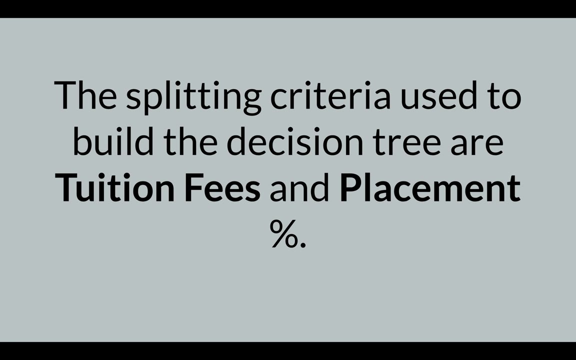 achieved, that is, you know, chosen by the decision tree, and then it will make that decision based on how Purely a splitting criteria is dividing the data set into classes. So let's say that our decision tree went through all the data, all the characteristics of the 100 universities. 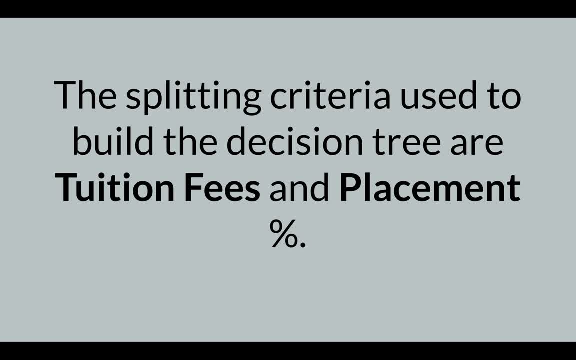 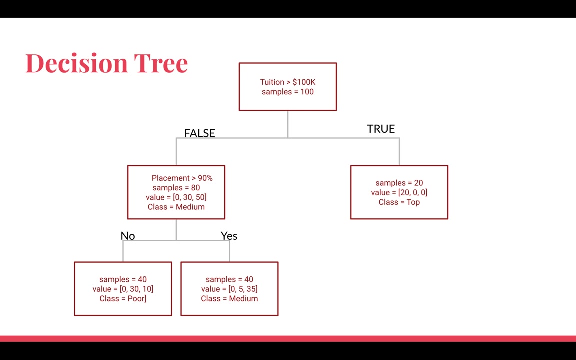 and found that tuition fees and placement are the two characteristics which are helping the decision tree algorithm to create really clean classification into the three classes of top, medium and poor. So this is our decision tree And here it's very similar to the way we saw the decision tree in the previous video. 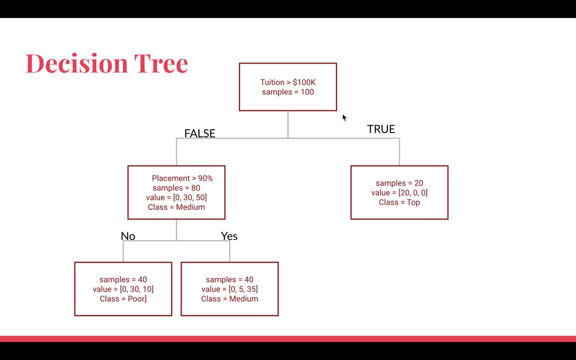 There's a little bit of change. So here is our first splitting criteria of tuition fees, And here is our first split happening into these two nodes. And then here is our second splitting criteria of placement percentage, And here is the second split that is happening into another two nodes. 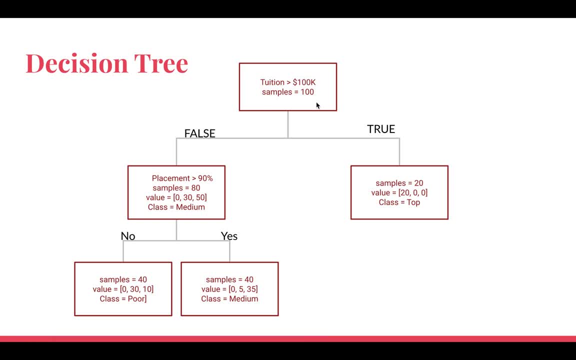 So let's understand them further. So here I have all the 100 samples and I'm checking whether tuition fee is greater than 100K or not. So all the samples Which satisfy this condition: that their tuition fee is more than 100K. 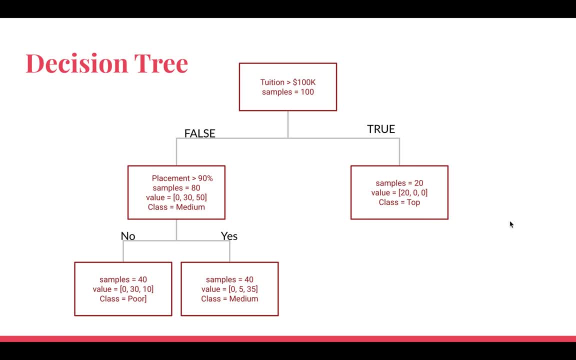 They come into this box. and let's assume that there are 20 such samples in my data set which have a fees of 100 or more than 100K. So here within the value square brackets, I have 20: 0, 0. So 20 means the 20 samples which belong to the class top rated. 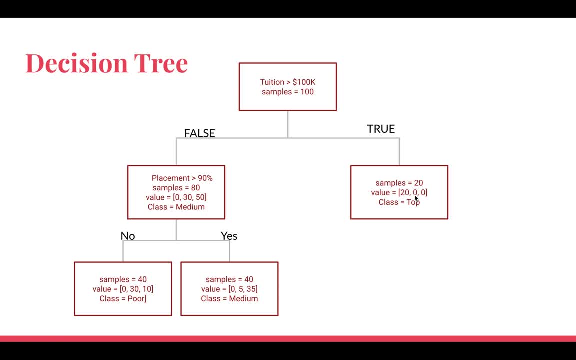 there are no University here which belong to either medium or poor. so this is what is: a pure node, whatever I have been referring to, because this node contains class of only one kind. it's not impure that, that is, it's not containing three types of data, three type of the classes within it. it is a pure node. it. 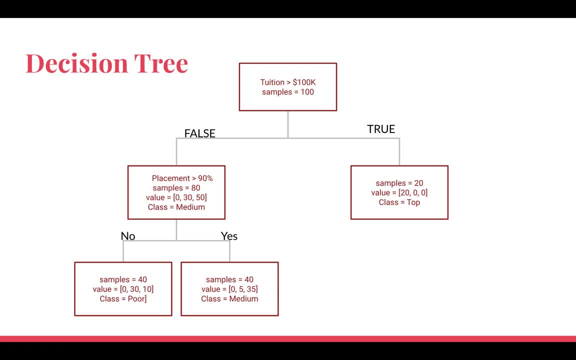 has cleanly classified these 20 universities to be belonging to the class top. okay, on the left hand side, if you see, here our node is not that pure. for the remaining 80 samples, 30 of them belong to class poor and 80 of them belong to class poor and 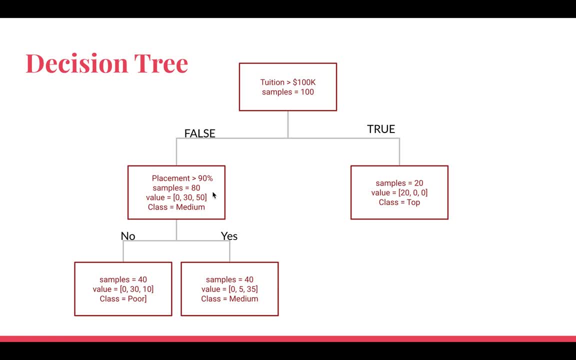 50 of them belong to the class medium, but because here medium is higher in number, so we call this node as a medium, because that's that's in majority. but if we further break it down, if we further split using placement greater than 90%, so in that case all the universities which have placement greater than 90%, so 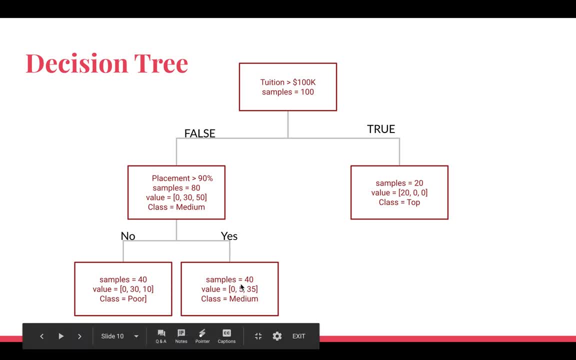 what we found is that 5 and 35- and this one is 0, top rated is 0, but there are 5 poorly rated and 35 medium rated universities that fall in this node and there are total 40 samples. and here also there are 40 samples. 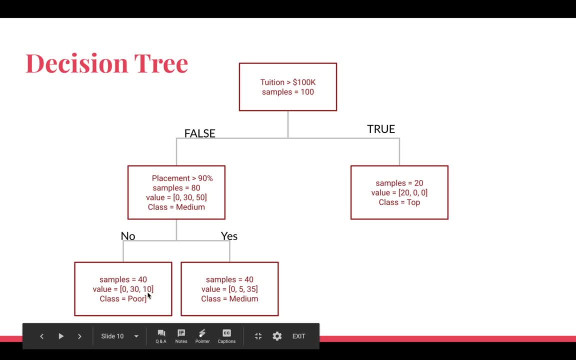 and 30 of them belong to the poor class and 10 of them belong to the medium class and, depending on the majority class, the node is assigned its final class. So this one is class poor and this one is class medium. So I hope you understand how this decision tree was formed and how each class was. 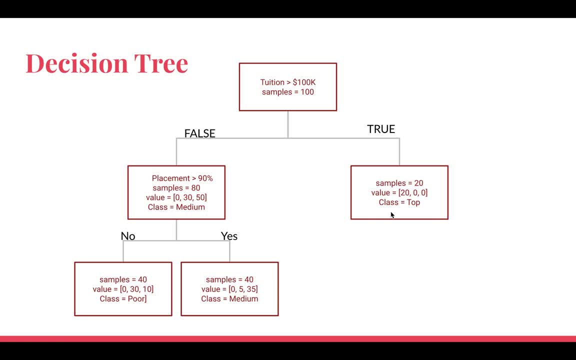 assigned to a particular node. Now, this node is a pure node because it contains samples belonging to one class only. but these two nodes are not that pure because, even though it is a pure node, it is not that pure because it contains samples belonging to one class. 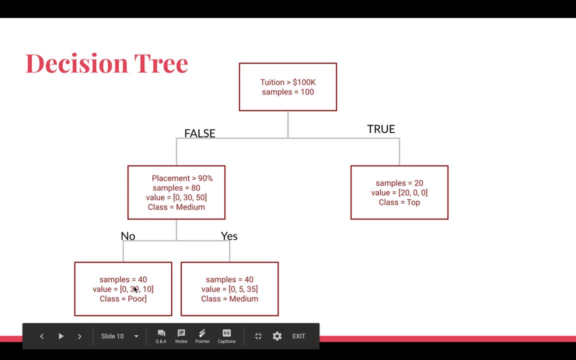 and even though we classify this as poor, because the poor rated universities are more here, but there are still 10 medium rated over here and here, even though there are 35 medium rated, but there are still 5 poor rated. So these are not pure. these don't contain the records or the 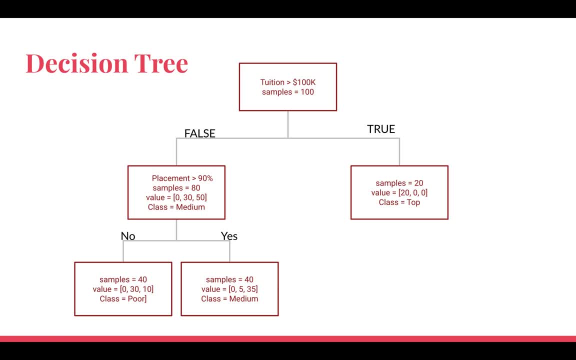 universities belonging to only one class. So these are impure nodes. So let's say, I want to calculate the Gini index of this highlighted node. So how do I do that? So it's very simple, and this is the formula for that: All I do is I take the total number of 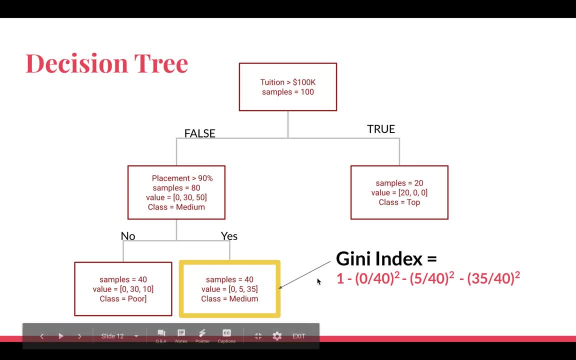 samples present in this node, which is 40 in this case, and I put that in the denominator and then in the numerator I put the number of records belonging to each class. So first one is 0, second one is 5 and third one is 35, and then I take the squares of that and then I subtract. 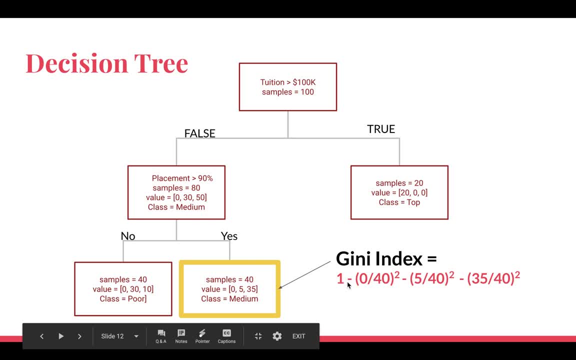 all of these from 1.. So that's the formula for calculating the Gini index, and when I complete the calculation, this is the number that I get: 0.21875.. Now, this number, although it is very, very low, it's still not 0, right, it's not a very pure. 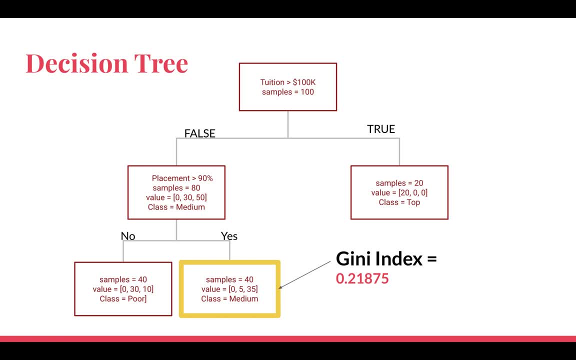 node. So you know, so we can decide based on the Gini index how good our node is and the decision tree while creating all these splits it is. it will actually calculate the Gini index of the nodes at each split for all the different features that are present and wherever it will find the minimum Gini index. that's the splitting criteria. 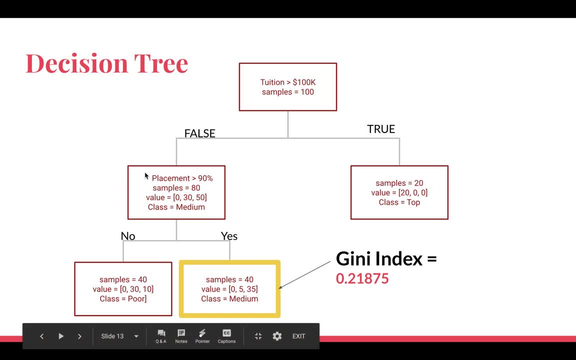 that it will choose So here instead of placement. maybe if it had used scholarship, then the Gini index of this node maybe it would have been 0.7 or something that is higher. So then it decided that, no, scholarship is not a good splitting criteria, because when I'm 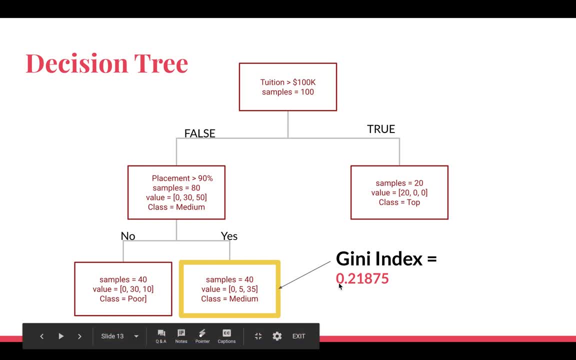 looking at a number like 1, it's a very low split, because it's a low split and if it is higher, then the dataset is very low as well. So here I'm taking using placement, I'm actually getting a lower Gini index right. so that's how the decision tree will.